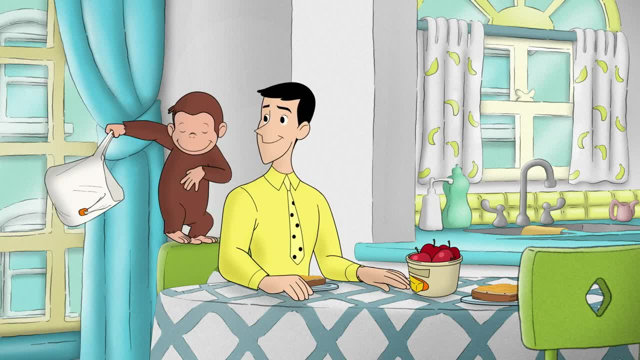 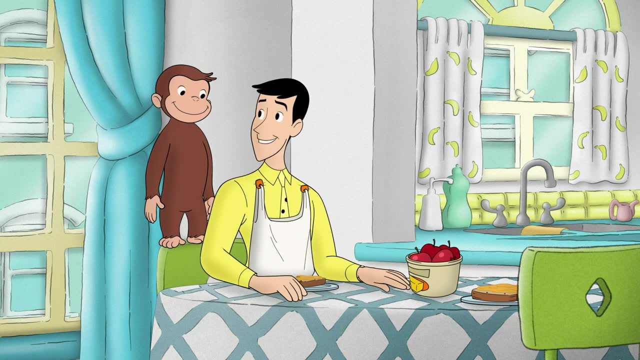 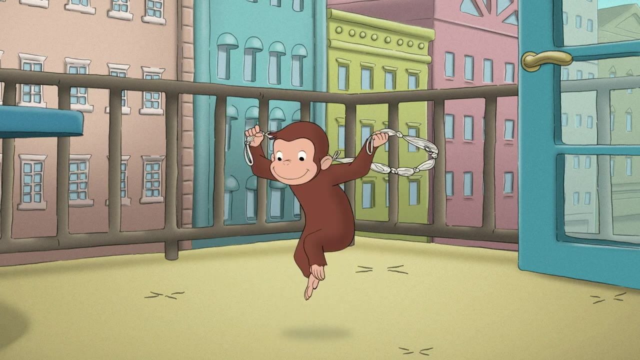 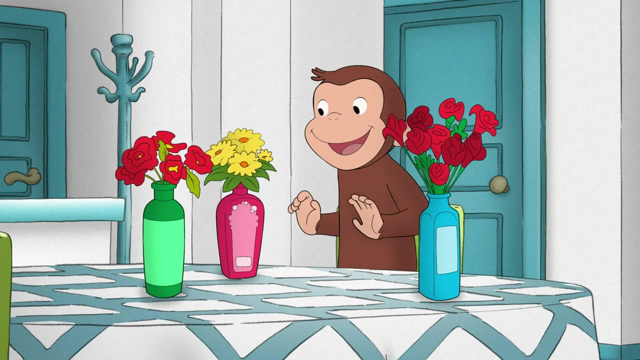 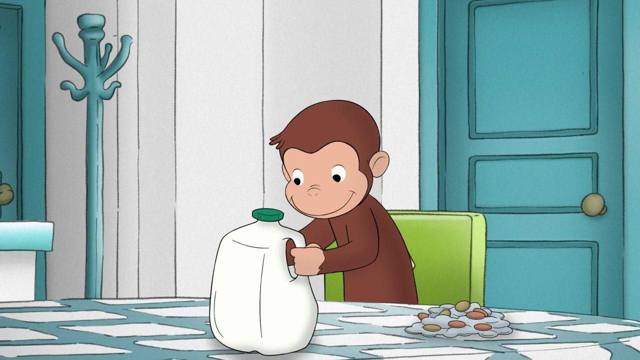 Ho-ho-ho-ho Ha A bib. Just what I needed. Thanks, George. George wondered what else he could make with plastic. Aww, Ha, Hmm, Hmm, Aww, He didn't look very comfortable. 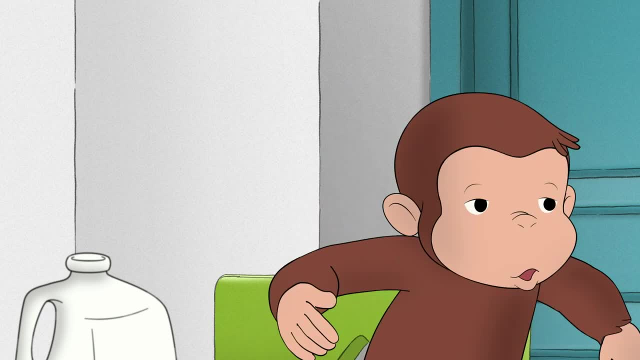 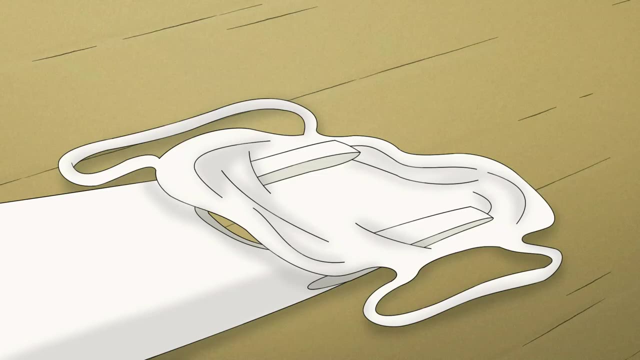 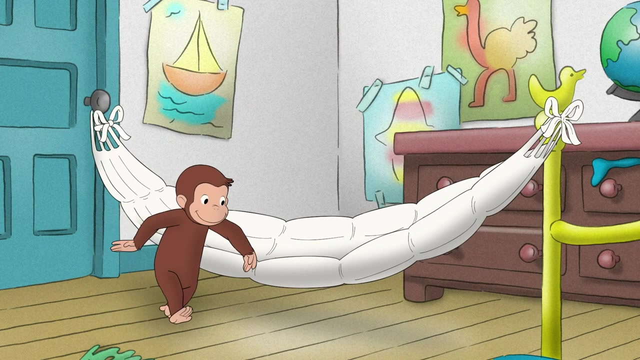 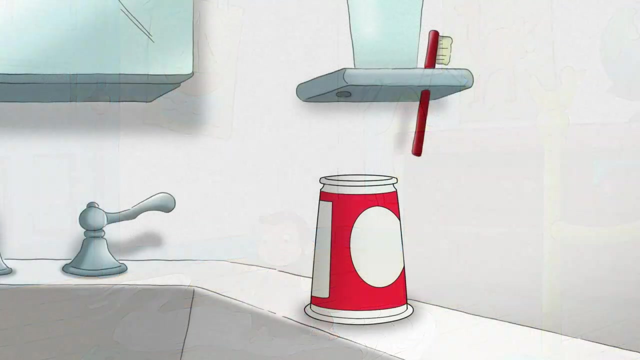 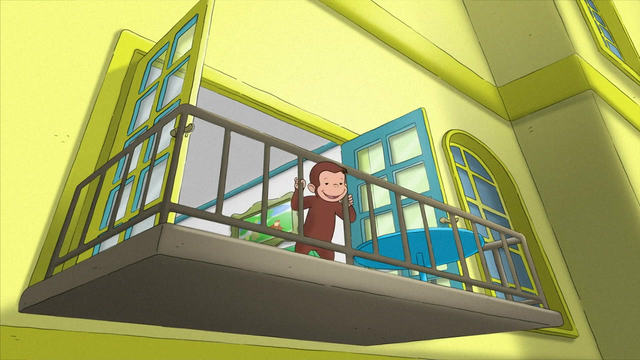 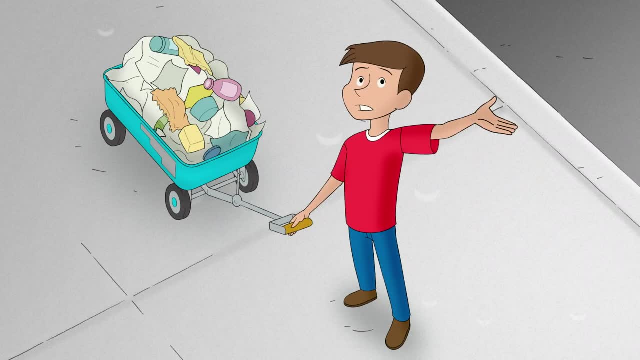 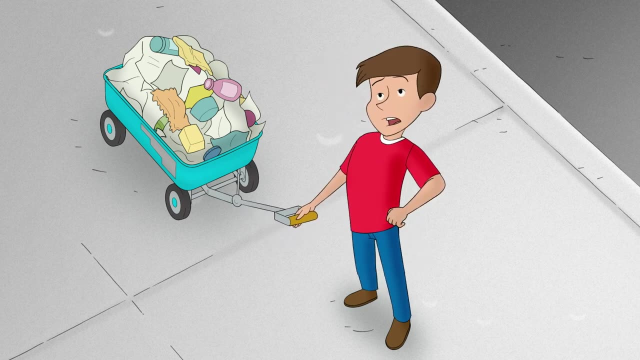 See all this plastic stuff. Since the day we saw that seabird stuck in plastic, I decided to never throw any plastic away ever. But Aunt Margaret said Enough is enough, It all has to go. So there's a store downtown that takes plastic stuff. 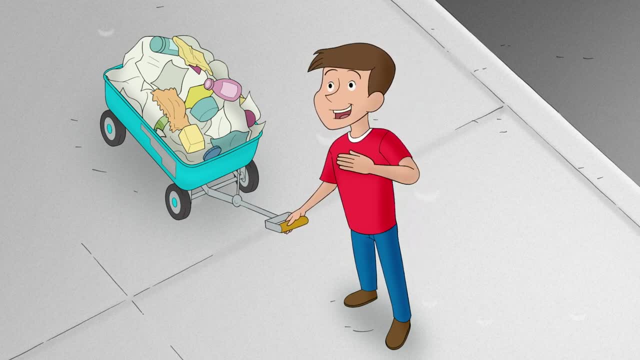 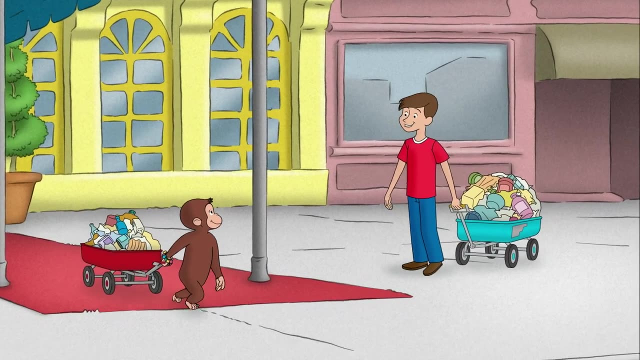 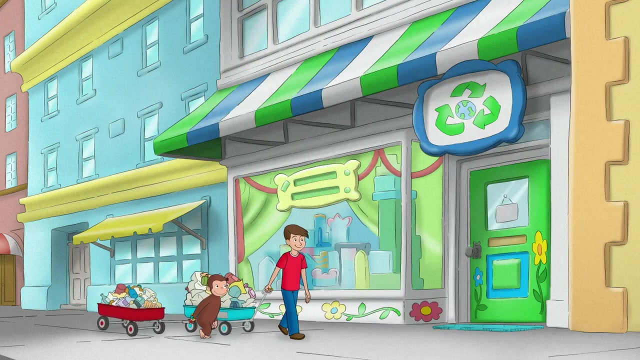 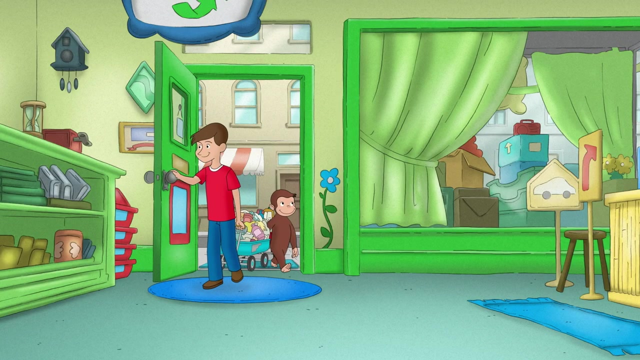 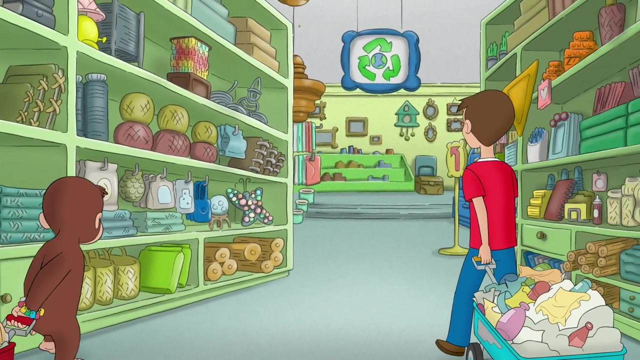 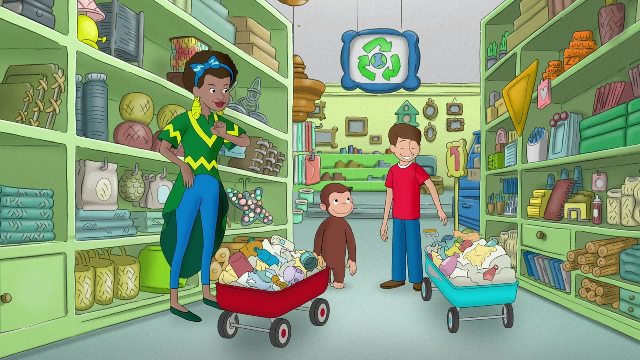 plastic, stuff that doesn't get recycled, want to go with me: reduce, reuse, recycle. I knew that is all that plastic for me. yep, it's all yours. awesome, I'll take all I can get. I use plastic that doesn't get recycled to make my odds and ends. wow, that's fantastic.